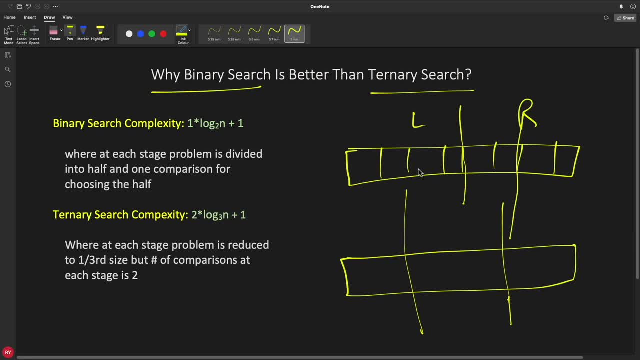 So, in each and every iteration, as we divide this binary search into two, in each and every iteration you will divide this into three. So, as you can see that you had this one comparison to decide whether you will go for the left one or the right one, 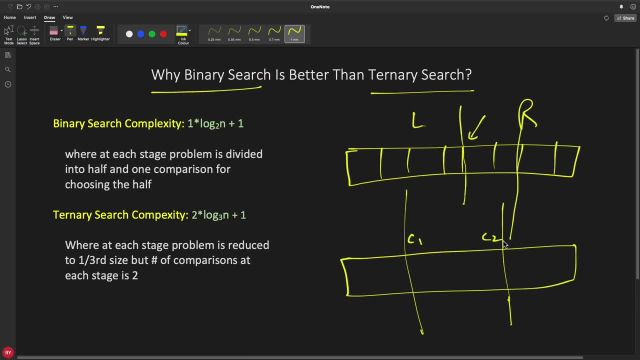 Here you have two In this comparison. you have two comparisons: This comparison one and this is comparison two. So every iteration you have two comparisons, whereas this is one comparison to choose. But here, good part is, you have one third space left, Whereas this is one by two. 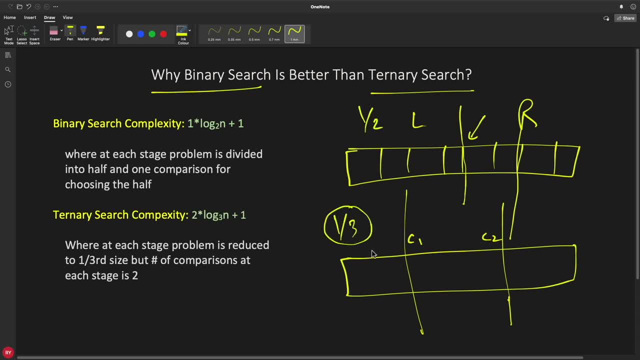 And this is very smaller, So you have very less space to search compared to this one, But still, I am telling you, binary search is more famous. You know that. So why? ternary sort is not good if it can divide space into one third, so let me erase this. so, as i told you that you have one comparison in binary search, 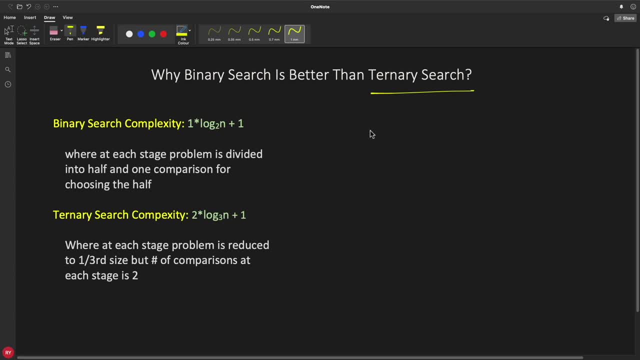 and two comparisons in ternary search. actually, if you look at the program you will find that in binary search you have two comparisons. one is actually you will compare whether the element is found or not. if it is found, then it is done otherwise, where you will go left or right. so 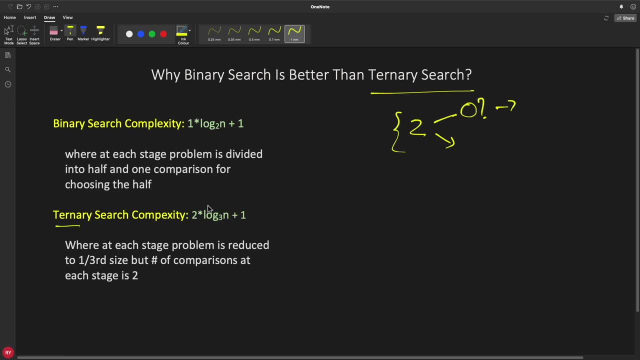 there are two comparisons, whereas in ternary search you have four comparisons. okay, so if i will write the formula for this, it would look something like this: we have two times log base, two n plus order of one. so this is for binary search, and for ternary search we have four cross. 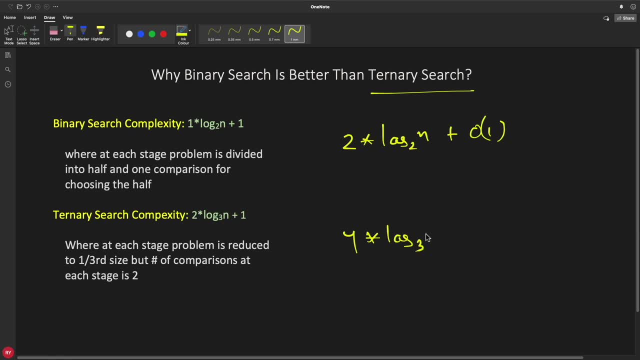 log three, because we are dividing space into three now and n plus order of one. so this order of one is like how much time you take to reach to some place, so that you can compare that with another. one is a constant time, like it's an array, so you can directly jump to that element and compare. so 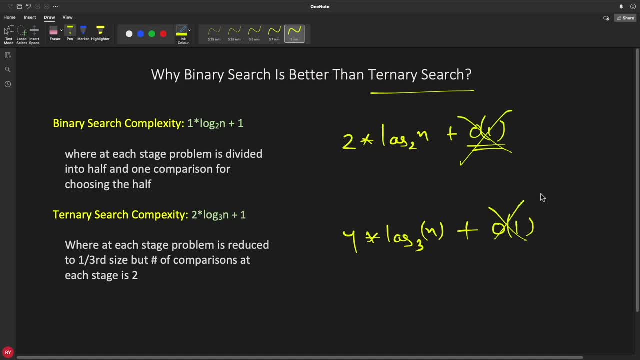 this is like not in the consideration. we can remove this. yeah, now, now you are going to compare these two. if you will do little bit of math, this would get converted into log two n and this will be like two log three n, and now we have to compare these two to come up with a solution, whether this is good or this is. 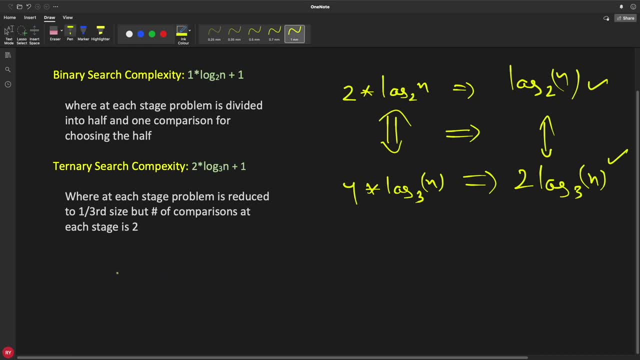 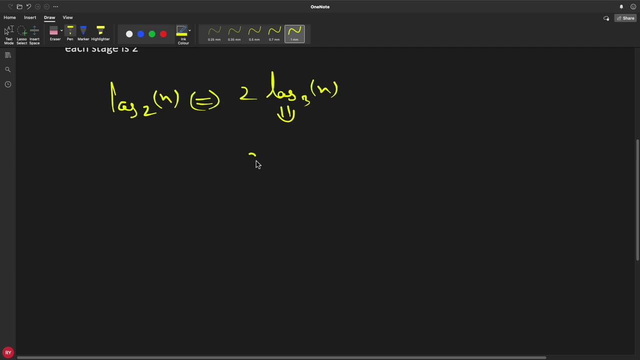 good. so let's try to compare these two. and what we are doing here is we are comparing log two n with two log three n. so this can be converted into something like this: we have two multiplied by log 2, divided by log 3, multiplied by log base 2, n. okay, now you are comparing this one. 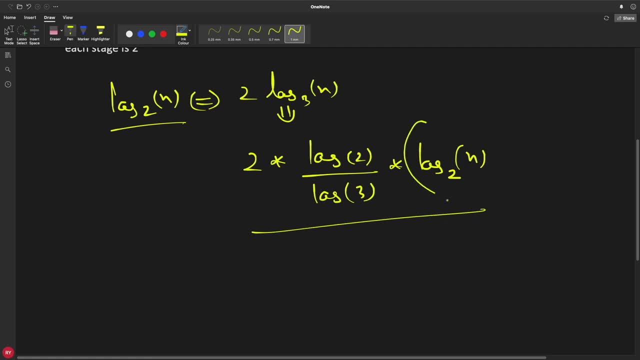 with this one. so these two elements are same meaning. you are going to compare this constant, so here we have nothing meaning. 1: 1 into this right and this is going to get compared with 1. it is obvious that this is greater than 1. if 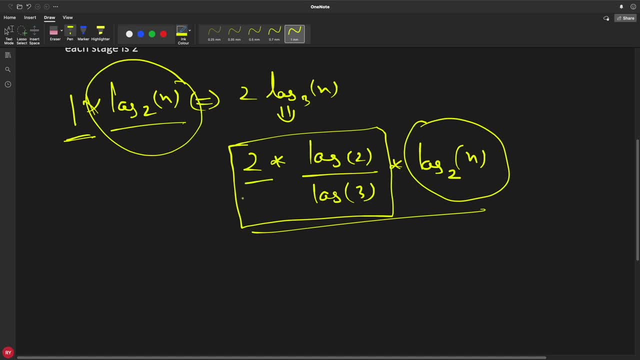 you calculate log 2 divided by log 3 multiplied by 2, you will get that. so it proves that this particular constant is greater than 1. that's why ternary sort is not good. the constant is playing a really very big role here, generally in 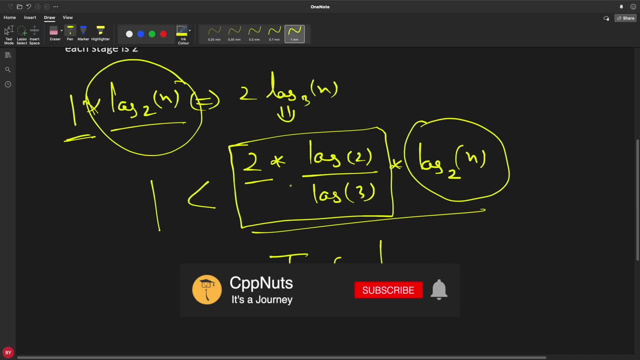 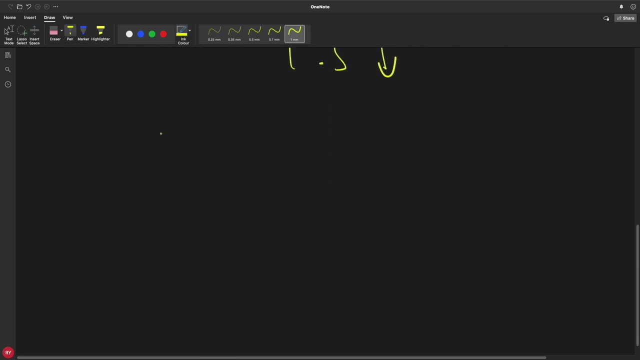 algorithm, computations and analysis. we don't care about the constants, right, but here it is really very important role-playing factor. so if I will tell you, you have to compare with log 2 to the power n and log 2, and with some number, X multiplied here and number Y multiplied by here, and Y is less than X. 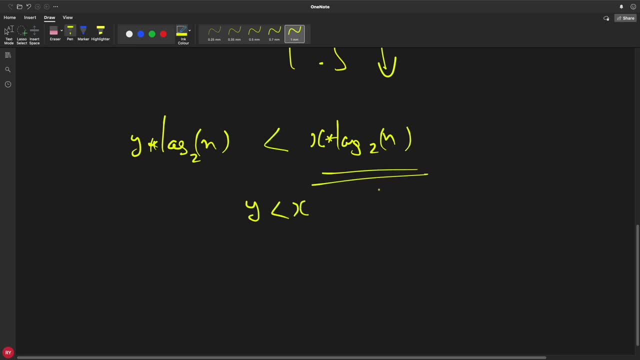 which one is taking more time. this one because X is greater than Y, meaning this is less than this. so that's why we always use- and there is a proof- that you divide your search space into half, then it is supposed to perform really very good as compared to dividing this whole thing into three or four, because we have 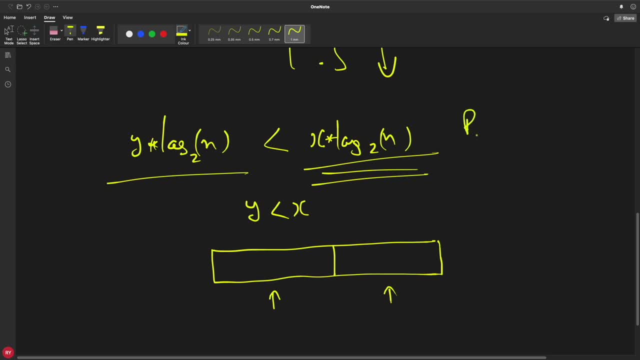 the options right, because when you write recursive functions, so you write like this, only like recursion, you will give first half here, so first half and second half will go here and then here you will do whatever the operations you want to do with those first half, second half. i mean. i'm just talking about the merge sort here, because that 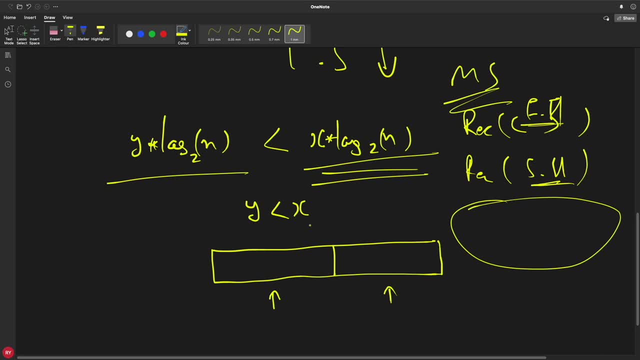 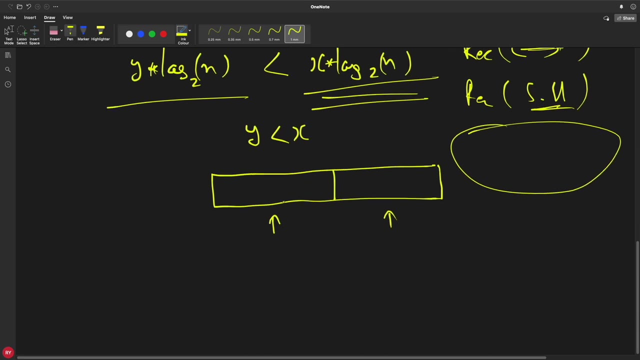 is very good example to explain this. so it is proved. i have not proved it. i have just proved that binary search is better than ternary search. and what i'm talking about is: there is a proof. i am not explaining that, but i have gone through that paper and i know that there is some proof. 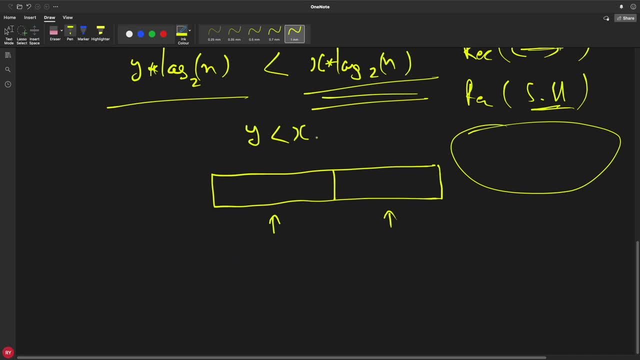 existing, which tells that if you will divide your space into half, exactly half, then it will perform way better than dividing your space into multiple spaces and then looking for the particular space. but you know what? actually, in algorithm world, you cannot say that one algorithm is good than. 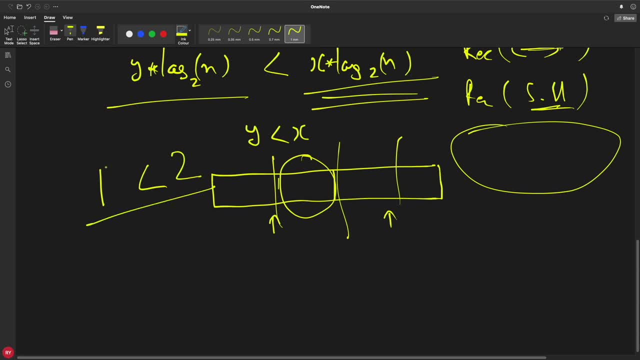 another algorithm. no, actually it depends. maybe this one algorithm is performing well good 99% of the time, but this is also good for 10%. and what is that 10%? you have to see the data and, most likely, what you will search all the time. so i hope you would have understood what i was. 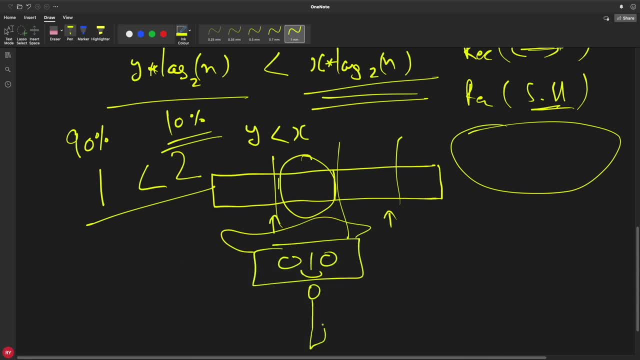 trying to explain here, so i'll see you in the next videos. bye, bye, take care. 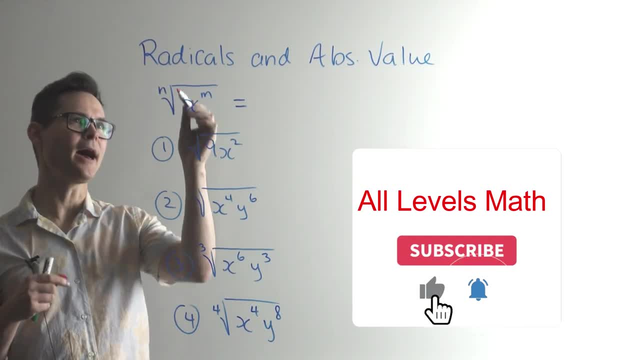 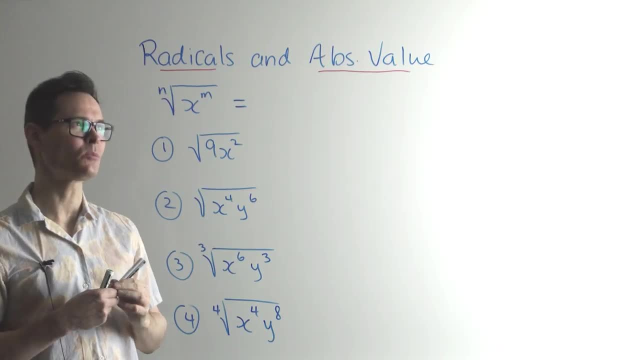 Welcome back to my channel. Today we're going to take a look at radicals and absolute value in the answer. If you're taking an enriched math course or more challenging one, your teacher may require you to know this, or sometimes teachers just sort of skip over this because it can be a little bit. 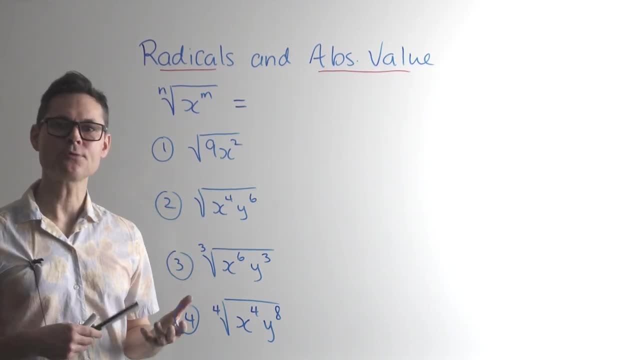 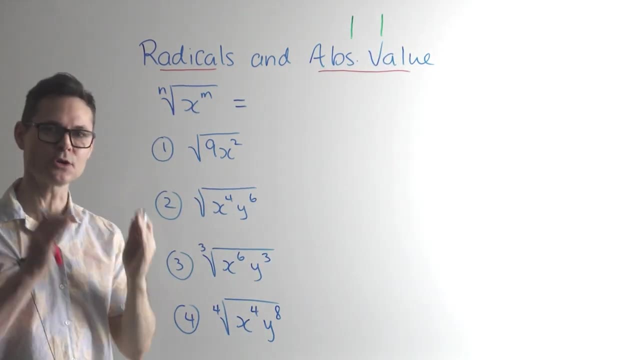 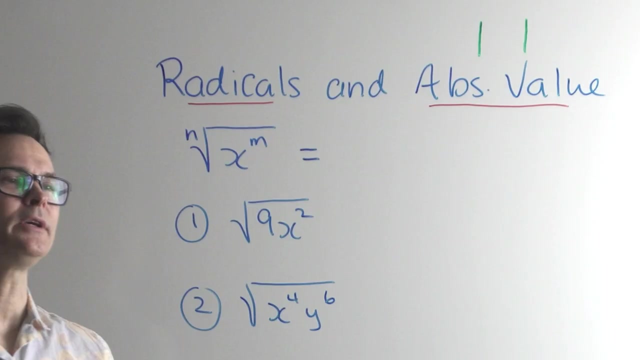 confusing to get into, But let's go through sort of the motivation for absolute value. making sure that you know absolute value is a set of brackets. They're vertical bars and we'll see what that means in a second. Okay, so radicals, Here is a radical. It looks ugly. 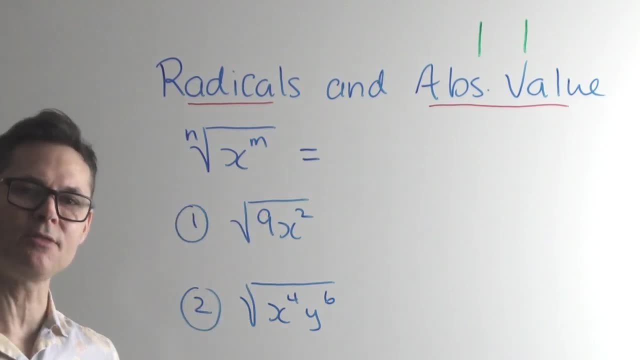 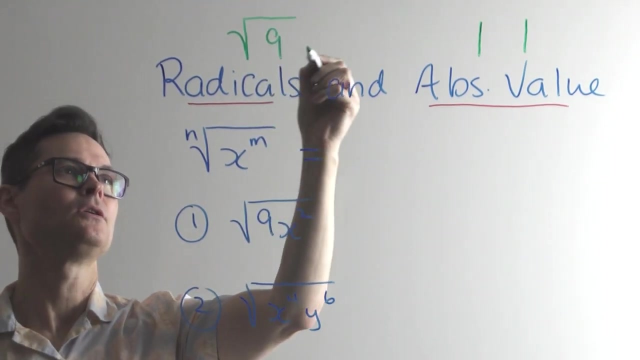 It's got a power on the inside, m- and it's got an nth root on the outside. And what we have to be careful with here is when you take, for instance, if I take- the square root of a number, say nine, then the idea here is that the square root is actually the.